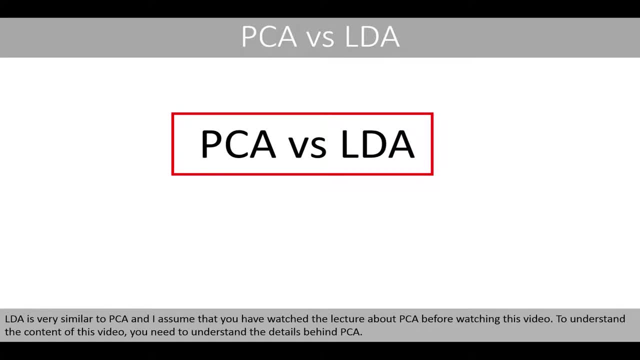 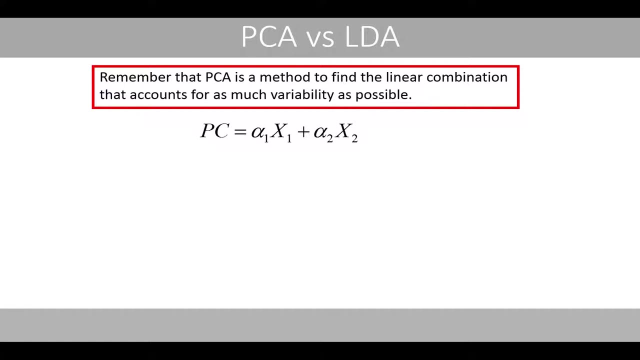 LDA is very similar to PCA and I assume that you have watched a video by PCA before watching this video. To understand the content of this video, you need to understand the details behind PCA. Remember that PCA is a method to find the linear combination that accounts for as much variability as possible. 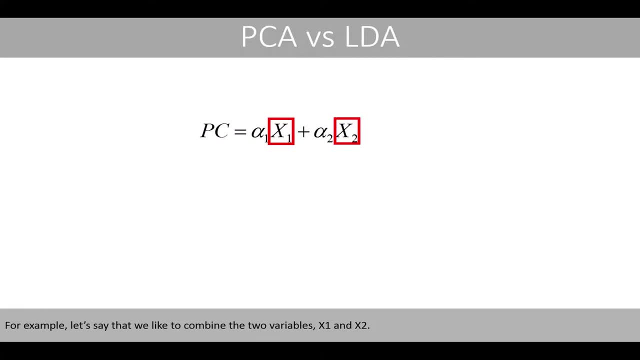 For example, let's say that we like to combine the two variables x1 and x2.. PCA will then try to find the optimal values for the weights alpha1 and alpha2, so that the combined variable has maximal variance. Remember that the values we use for the weights are constrained so that the sum of the squared weights is equal to 1.. 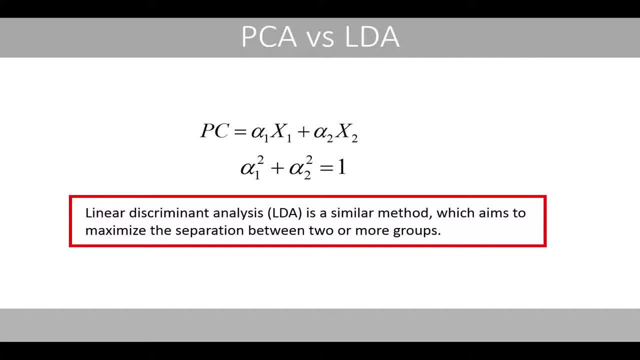 LDA is a similar method which aims to maximize the separation between two or more groups. Let's say that we like to combine the two variables x1 and x2.. LDA then combines these two variables by using optimal values of the weights so that the combined variable shows maximal separation between the groups. 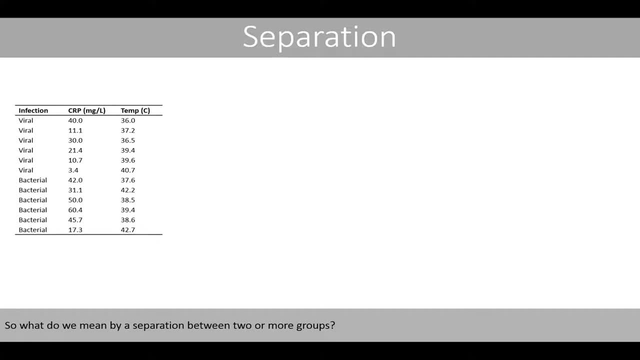 So what do we mean by separation between two or more groups? To explain separation, let's have a look at the following fictive dataset: Let's have a look at the following fictive dataset: Let's have a look at the following fictive dataset: 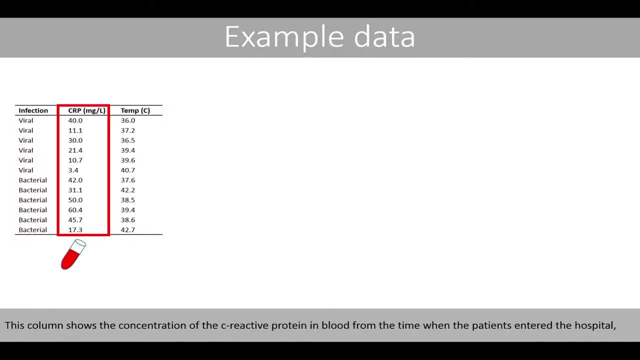 This column shows the concentration of serorheactyl in blood from the time when the patients entered the hospital, whereas this column shows the body temperature of the same patients at the same time point. Once the patient had entered the hospital, the presence of bacteria and virus were analyzed from different samples. 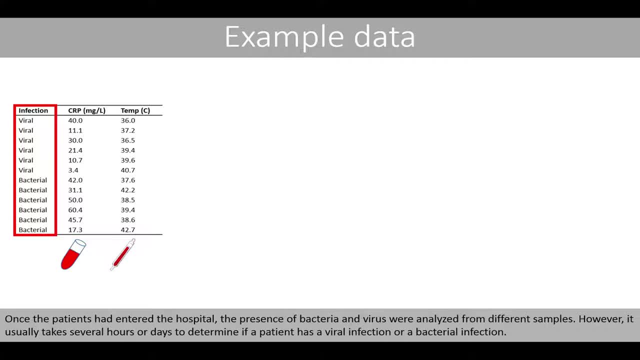 However, it usually takes several hours or hours to analyze the presence of bacteria and virus from different samples days to determine if a patient has a viral infection or bacterial infection. after two days at the hospital, these six patients were found to have a viral infection, whereas these six patients were confirmed to have a bacterial 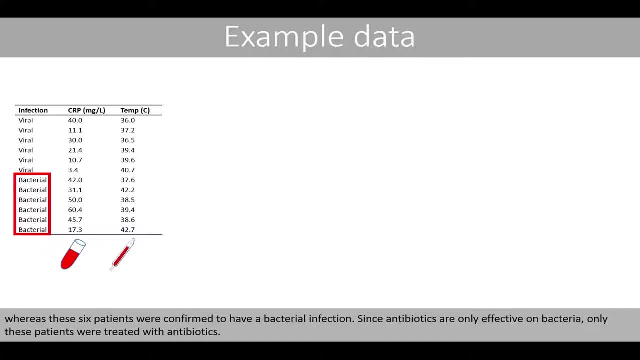 infection. since antibiotics are only effective on bacteria, only these patients were treated with antibiotics. the problem is that we have to wait two days to know if antibiotic treatment is appropriate or not. it will be nice if you could use the CRP concentration or the body temperature to tell if a 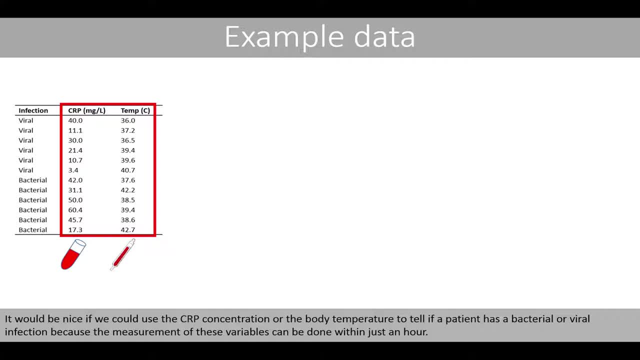 patient has a bacterial or viral infection, because the measurement of these variables can be done within just an hour. if you plot the CRP concentration of the 12 patients, we can see that the ones with a viral infection nearly have a lower concentration of the CRP compared to the ones who have a 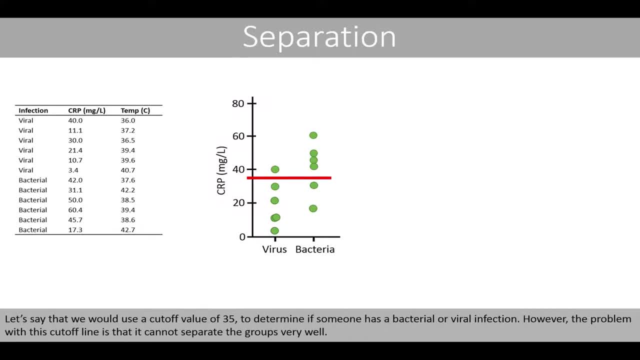 bacterial infection. let's say that we use a cutoff value of 35 to determine if someone has a bacterial or viral infection. however, the problem with this cutoff line is that it cannot separate the groups very well. we can see that four patients with bacterial infection and one patient with viral infection are above this line, whereas 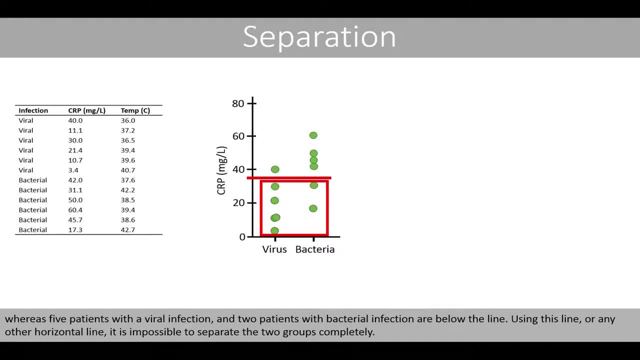 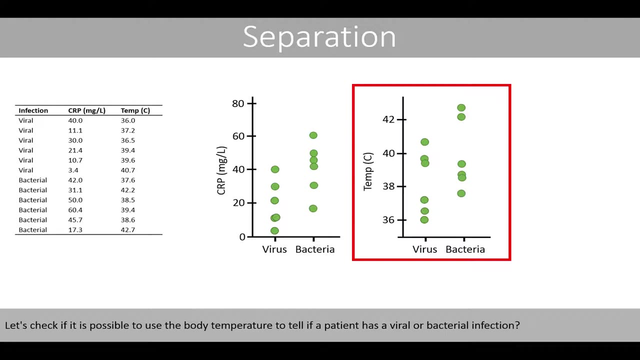 five patients with a viral infection and two patients with bacterial infection are below the line. using this line or any other horizontal line, it is impossible to separate the two groups completely. let's check if it is possible to use the body temperature to tell if a patient has a viral bacterial infection. as you see, we have the same problem. 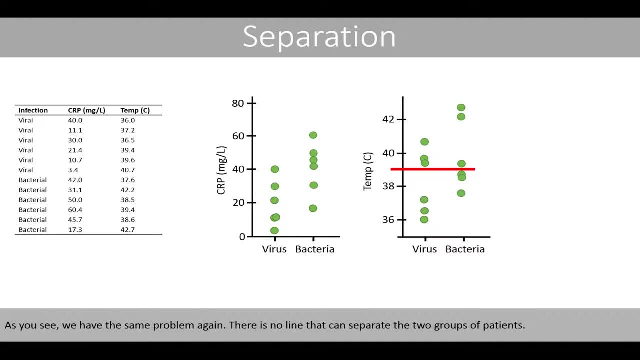 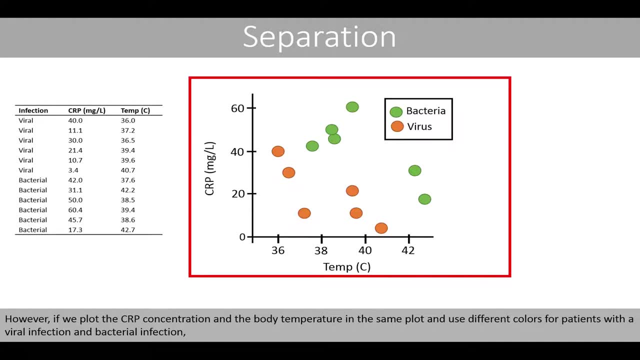 again, there is no line that can separate the two groups of patients. however, if we plot the CRP concentration and the body temperature in the same plot and use different colors for patients with a viral infection and bacterial infection, we can see that the following line can separate the two: 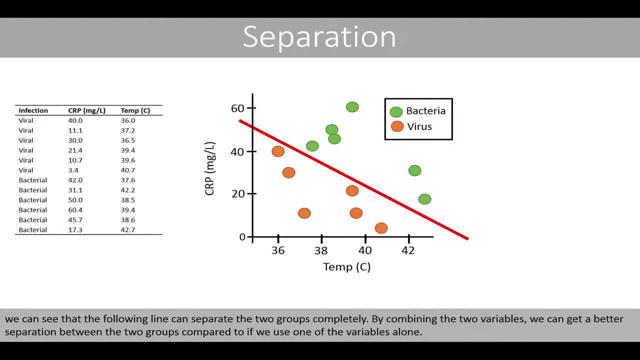 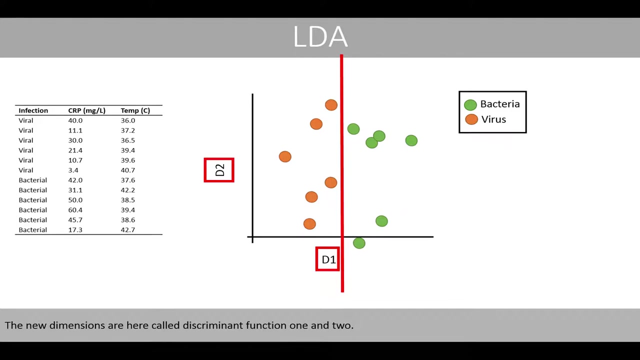 groups completely. by combining the two variables we can get the better separation between the two groups compared to if we use one of the variables alone. just as PCA, LDA can be seen as we rotate the data into two new dimensions like this. the new dimensions are helical, discriminant function one and two. we 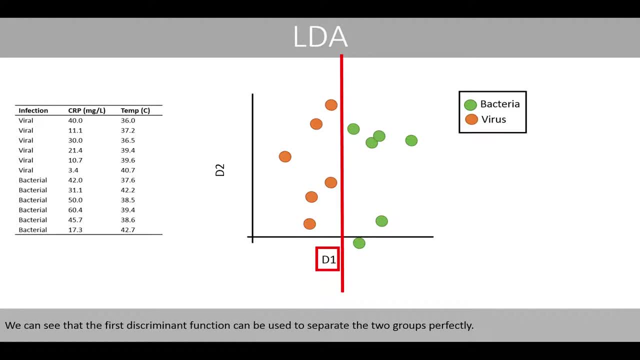 can see that the first discriminant function can be used to separate the two groups perfectly. in contrast, we cannot separate the groups based on the horizontal line, which means that the second discriminant function is not useful for separation. we can therefore delete the second discriminant function and place all data. 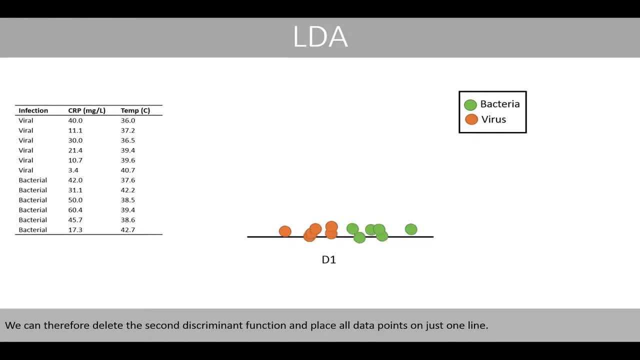 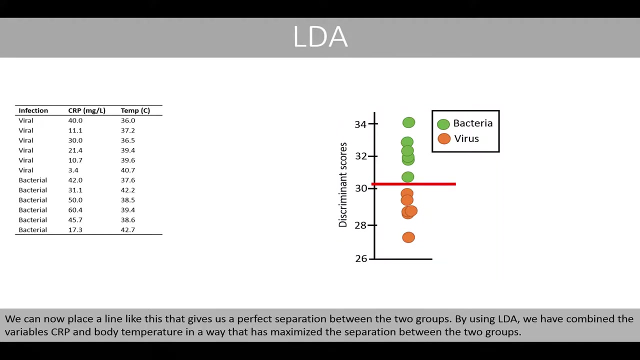 points on just one line. for illustrative purposes, we here rotate the plot so that the data points are plotted vertically. if you use LDA, we can plot the so-called discriminant scores like this. we can now place a line like this that gives us a perfect separation between the two groups. by using LDA, we have combined the 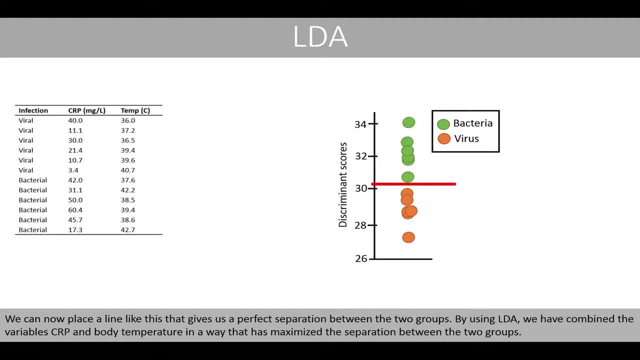 variable CRP and body temperature in a way that has maximized the separation between the two groups. the linear discriminant scores that you see in this plot can be obtained by the following equation: we can replace x1 and x2 with a variable names CRP and temp. 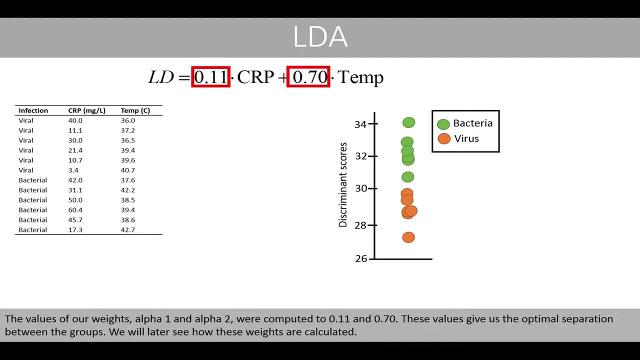 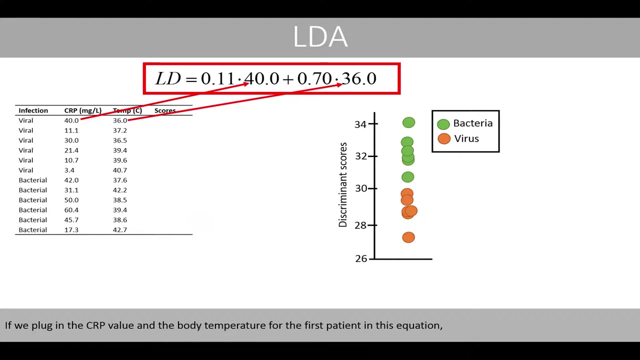 the values. our weights, alpha 1 and alpha 2, are computed to 0.11 and 0.7. these values give us the optimal separation between the groups. we will later see how these weights are calculated. let's use this equation to calculate the discriminant scores. if we bag in the CRP value and the body temperature for the 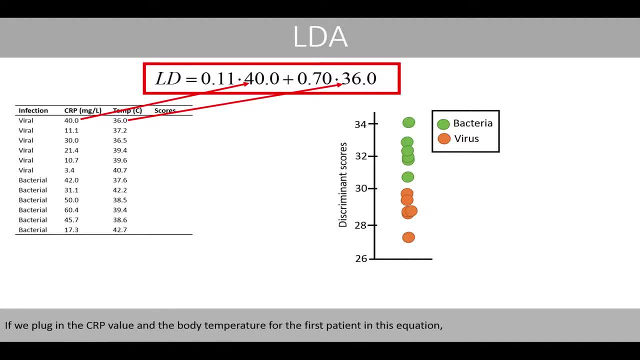 first patient. in this equation we see that the corresponding discriminant score is about 29.5. this score is represented by the following point in the plot: we use the same equation to compute the scores for the other patients as well. we can see that the scores for the ones with a viral infection are lower compared to the ones 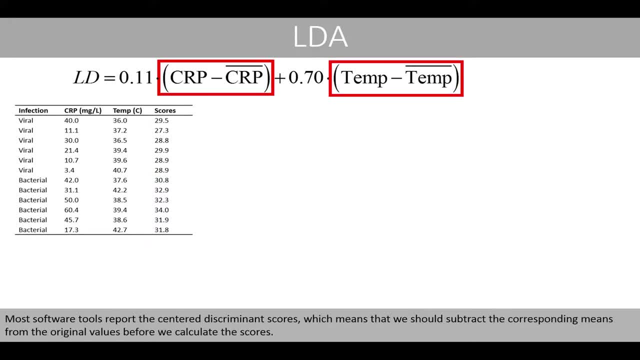 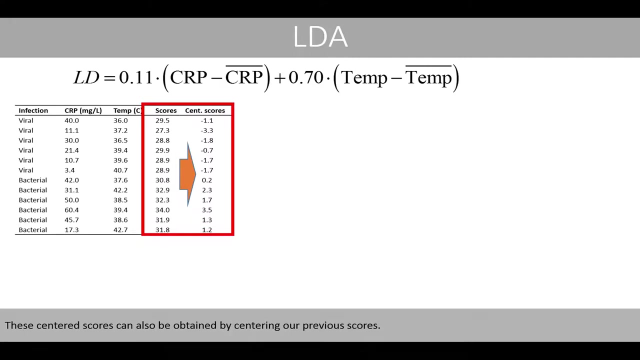 who have a bacterial infection. most software tools report the center discriminant scores, which means that we should subtract the corresponding means from the original values before we calculate the scores. by using this equation, the following centered scores were calculated: these centered scores can also be obtained by centering our previous scores. 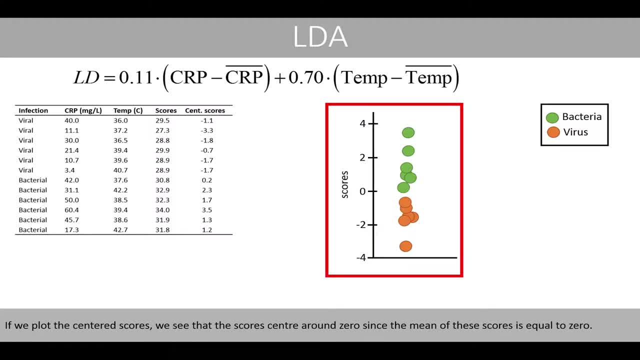 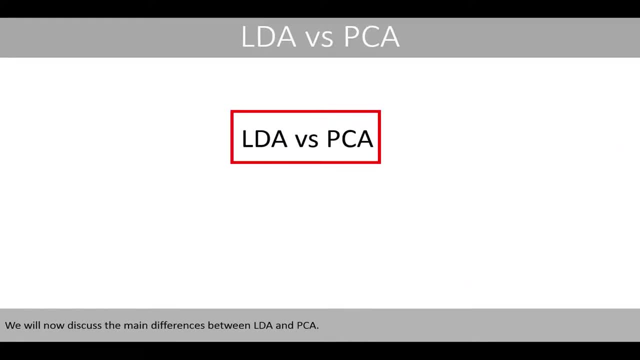 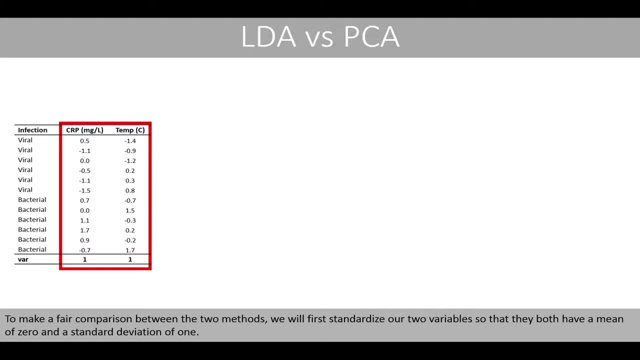 if you plot the centered scores, we see that the scores center around zero, since the mean of these scores is equal to zero. we'll now discuss the main differences between LDA and PCA. to make a fair comparison between the two methods, we will first standardize our two variables. 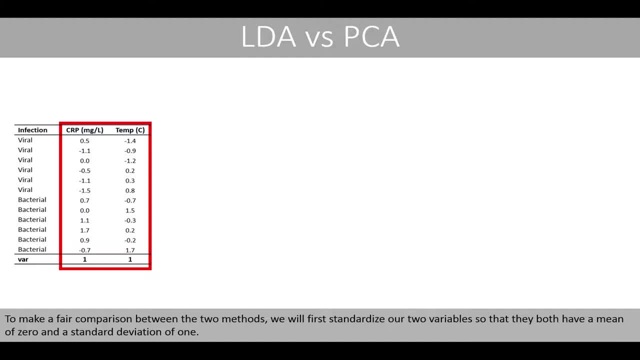 so that both have a mean of zero and a standard deviation of one. remember that we can standardize a variable by the following formula: or we subtract the mean from the values of that variable and divide by the standard deviation. for example, this first standardized value has been: 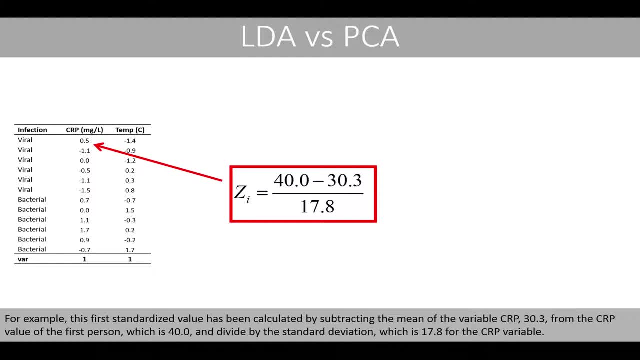 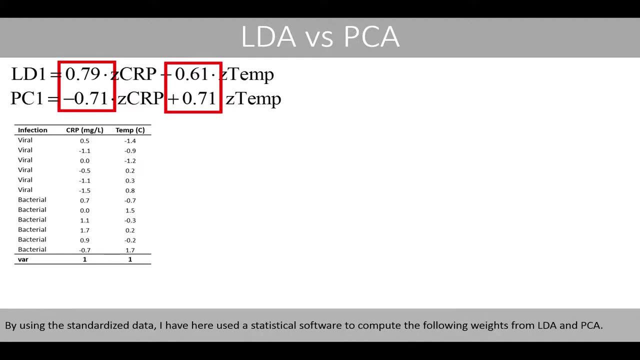 calculated by subtracting the mean of the variable, CRP 30.3, from the crp value of the first person, which is 40.0, and divide by the standard deviation, which is 17.8, for the CRP variable. by using the standardized data here used the: 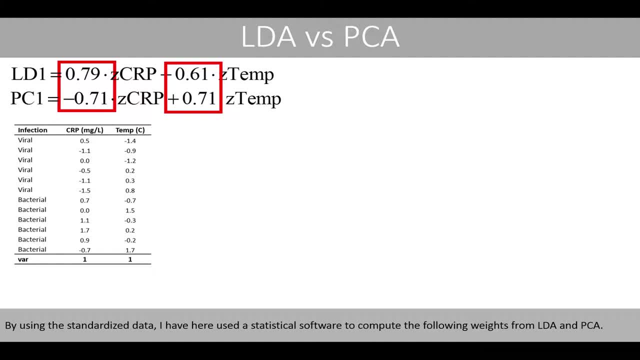 statistical software to calculate the following weights for LDA and PCA. Note that the variables represent standardized variables with a mean of 0 and a standard deviation of 1.. By using a software, the following weights were extracted from the first eigenvector: 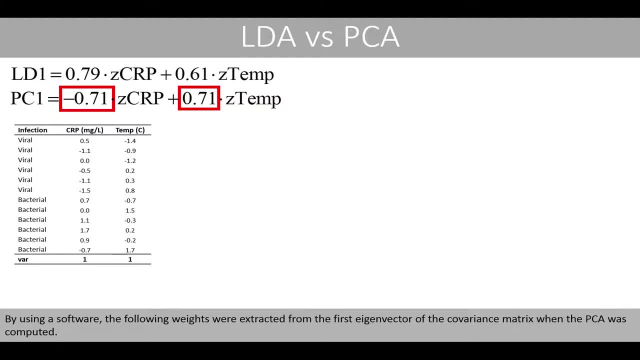 of the covariance matrix when the PCA was computed. These weights from the LDA were also extracted from the first eigenvector. However, this eigenvector is not an eigenvector of the covariance matrix. Instead, it is an eigenvector of another type of a matrix that we will discuss later. 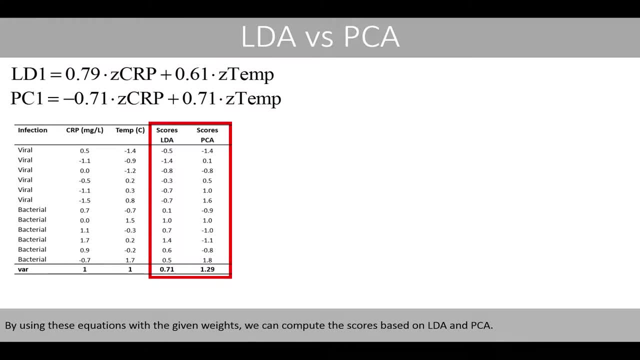 By using these equations with the given weights, we can compute the scores based on LDA and PCA. Note that the variance of the scores for the first principal component is 1.29, but only 0.71 for the scores based on the first discriminant matrix. 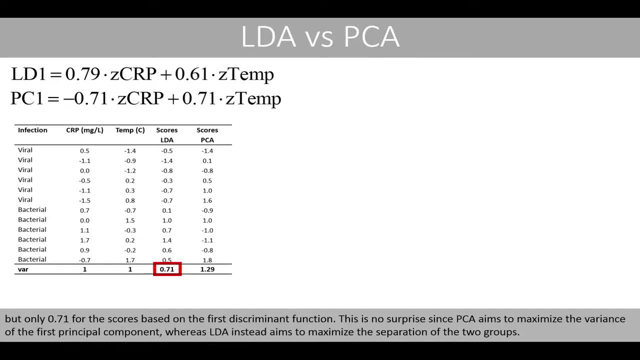 This is no surprise, since PCA aims to maximize the variance of the first principal component, whereas LDA instead aims to maximize the separation of the two groups. If we plot the scores computed by LDA, we see that the scores for the bacteria group 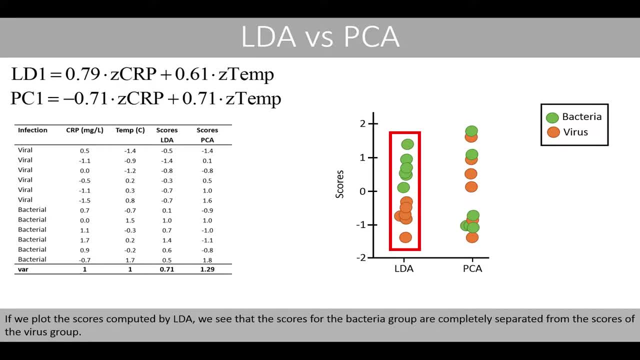 are completely separated from the scores of the virus group. In comparison, the scores computed by the PCA show no clear separations. The scores for the bacteria group are completely separated from the scores of the virus group. This is no surprise, since PCA aims to maximize the separation of the groups. 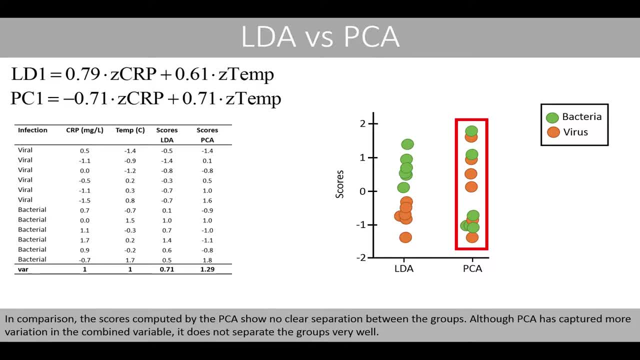 In contrast, PCA will not provide any separation between the groups. Although PCA has captured more variation in the combined variable, it does not separate the groups very well. Note that when we run PCA, we will not use this grouping variable at all, whereas in 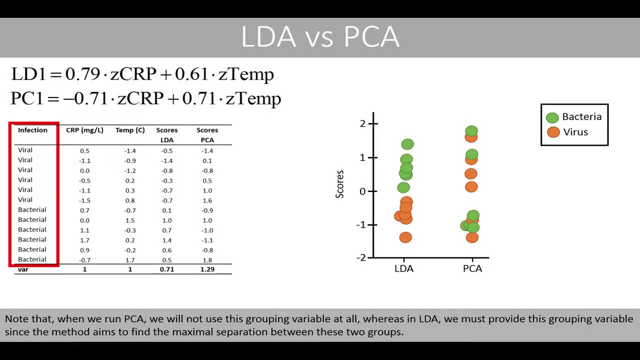 LDA. we must provide this grouping variable since the method aims to find the maximum separation between these two groups. Since PCA will only be based on these two variables, So we can't separate the groups anymore information about the groups, it will not be as effective as LDA in separating the 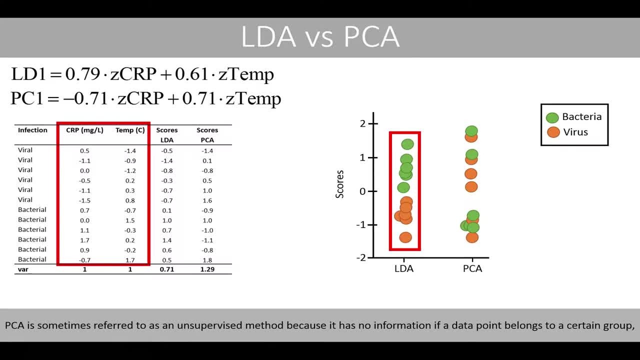 groups. PCA is sometimes referred to as an unsupervised method because it has no information if a data point belongs to a certain group, Whereas LDA is referred to as a supervised method because it has the information about which group the data point belongs to, in order to find the best separation between the groups. 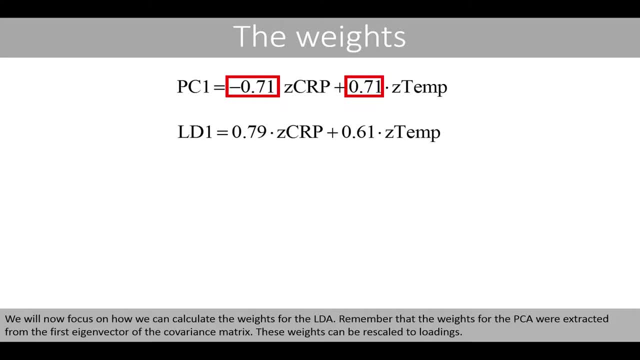 We'll now focus on how we can calculate the weights for the LDA. Remember that the weights for the PCA were extracted from the first eigenvector of the covariance matrix. These weights can be rescaled to loadings. The weights in LDA. 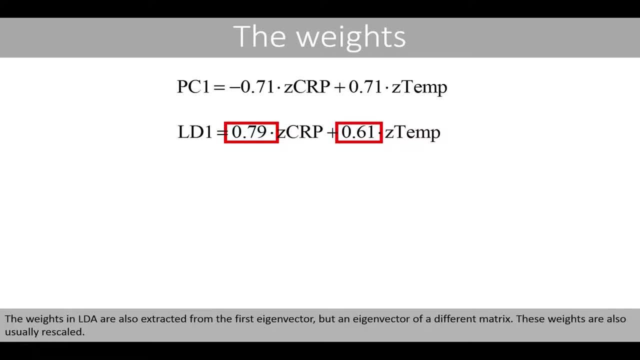 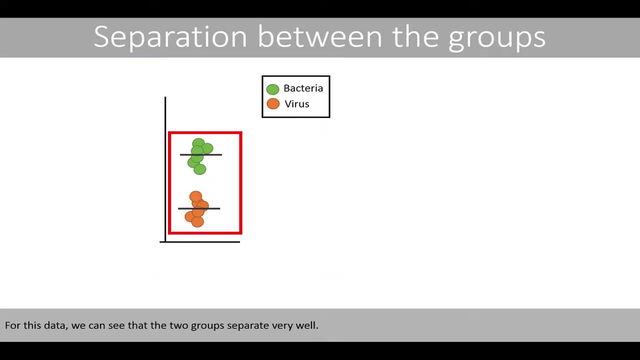 are also extracted from the first eigenvector, but an eigenvector of a different matrix. These weights are also usually rescaled. Let's first have a look at the LDA. LDA determines how well two groups are separated. For this data, we can see that 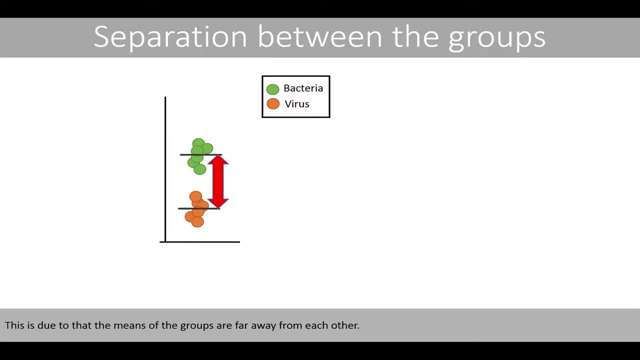 the two groups separate very well. This is due to that the means of the two groups are far away from each other. If the means are closer to each other, we can no longer see a clear separation between the two groups. The second reason why these two groups show a good separation. 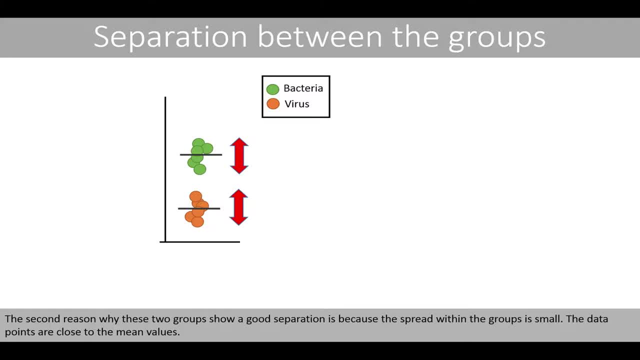 is because the spread within the groups is small. The data points are close to the mean values. However, if there is a much larger spread of observations around the means, then there is no longer clear separation between the groups, even though the difference in their means stay the same. If you calculate a grand, 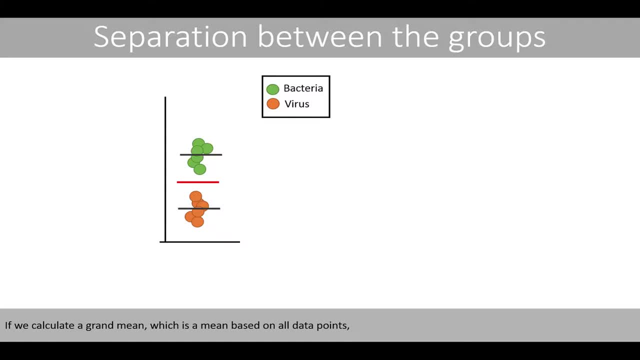 mean, which is a mean based on all data points. We can think of these distances as how much the group means varies from the grand mean. If the means are close, the variation of the group means around the grand mean is small, And if the two means are far away from each other, there will be a large variation of the 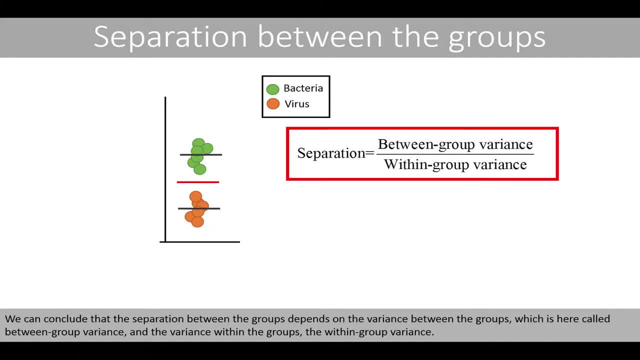 group means around the grand mean, We can conclude that the separation between the groups depends on the variance between the groups, which is here called between-group variance, and the variance within the groups. Note that this ratio is similar to the ratio used for ANOVA To get a good separation. 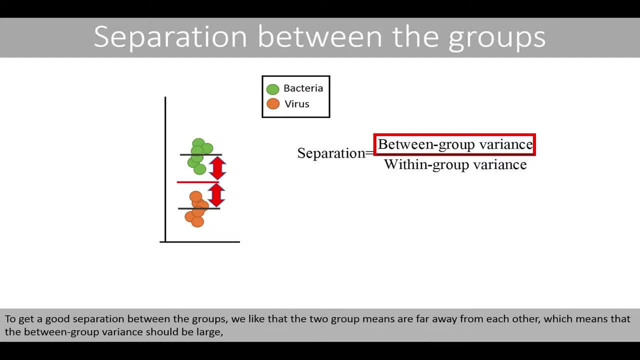 between the groups. we like that. the two group means are far away from each other, which means that the between-group variance should be lower large And the variation within the group should be small, which will result in a low value of the within-group variance. Thus, the ratio of these measures should: 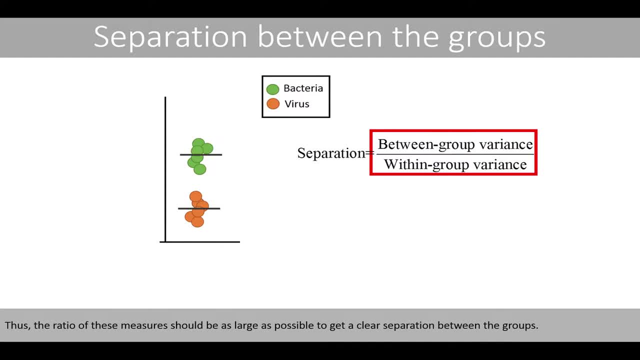 be as large as possible to get a clear separation between the groups. LDA combines variables based on this ratio where the aim is to transform the data so that the between-group variance is increased and the within-group variance is reduced. In matrix 4,, the separation can be described like this: where B is: 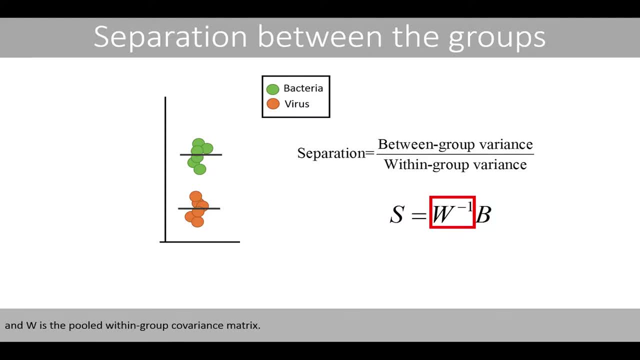 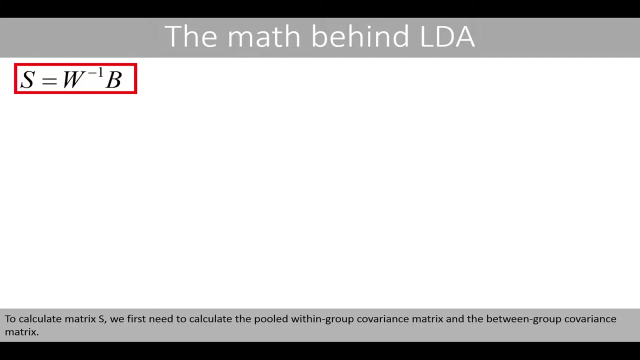 the between-group covariance matrix and W is the pooled within-group covariance matrix. Matrix S is our target matrix. We'll compute the eigenvectors of this matrix in order to get our weights To calculate matrix S, we first need to calculate the pooled within-group covariance matrix and the between-group. 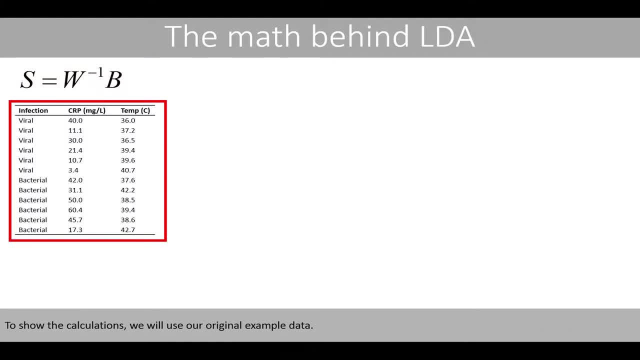 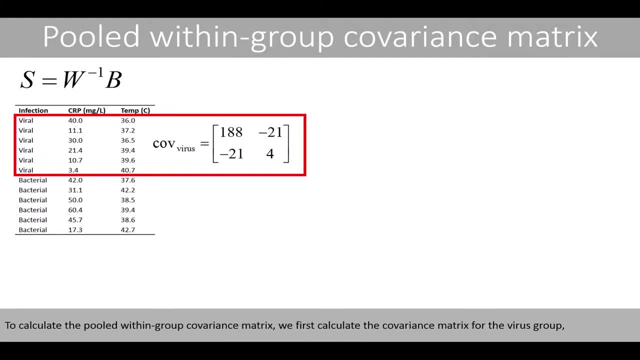 covariance matrix. To show the calculations, we'll use our original example data To calculate the pooled within-group covariance matrix. we first calculate the covariance matrix for the virus group And then for the bacteria group. Note that the values in these two matrices have 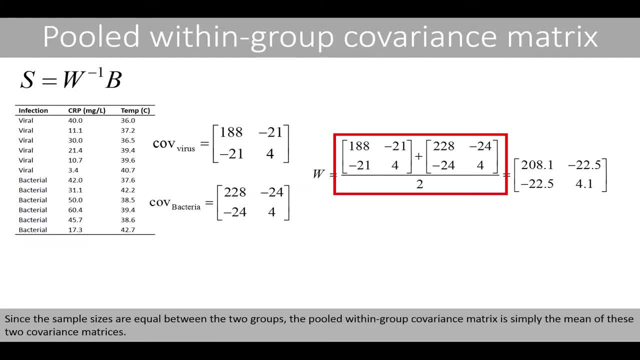 been rounded. Since the sample sizes are equal between the two groups, the pooled within-group covariance matrix is simply the mean of these two covariance matrices. If the two groups have an unequal sample size, we should use the following equation to compute the weighted average of the two covariance: 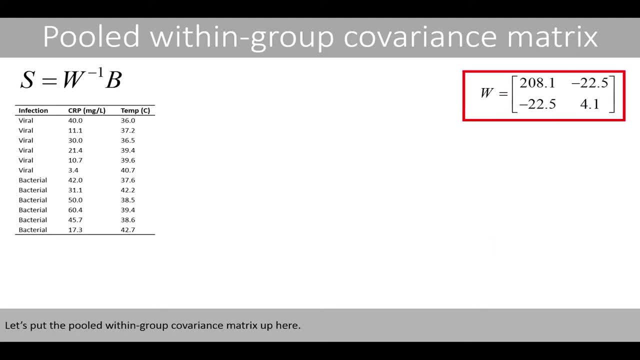 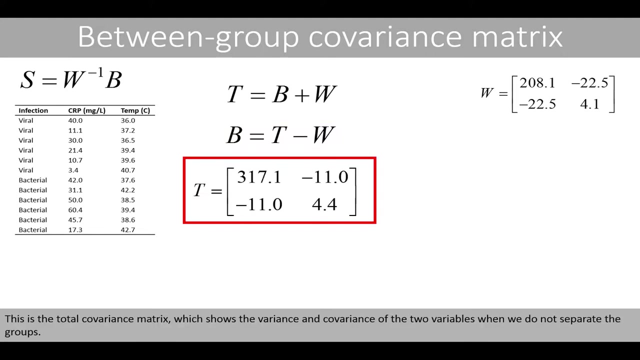 matrices. Let's put the pooled-within-group covariance matrix up here. We'll now try to calculate the between-group covariance matrix. A simple way to calculate the between-group covariance matrix is to first calculate the total covariance, because the between-group covariance is equal to the total covariance minus the pooled-within-group covariance. 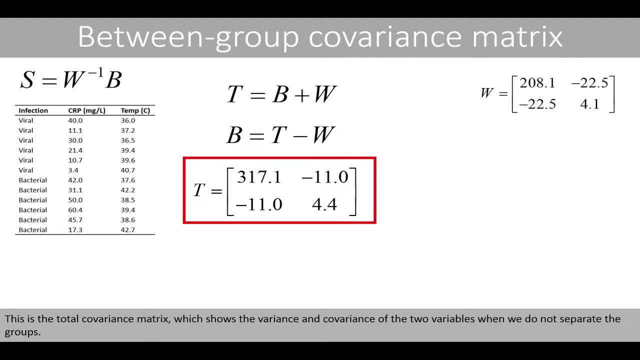 This is the total covariance matrix, which shows the variance and the covariance of the two variables when we do not separate the groups. The total covariance matrix is therefore the covariance matrix based on all data points. This matrix is the same covariance matrix that was used in the previous lesson For the covariance matrix. the covariance matrix. 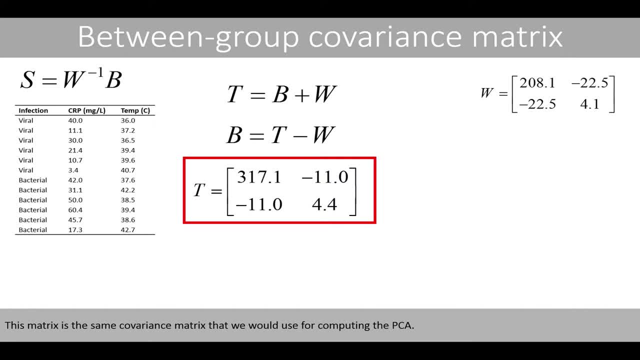 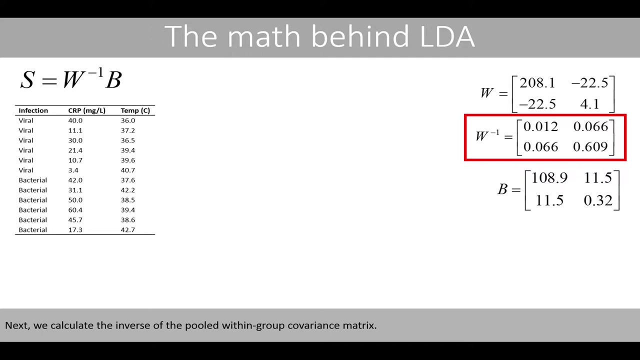 that we would use for computing the PCA. We can now calculate the between-group covariance matrix by subtracting the pooled within-group covariance matrix from the total covariance matrix. Let's put the between-group covariance matrix here. Next we calculate the inverse of the pooled within-group covariance matrix. 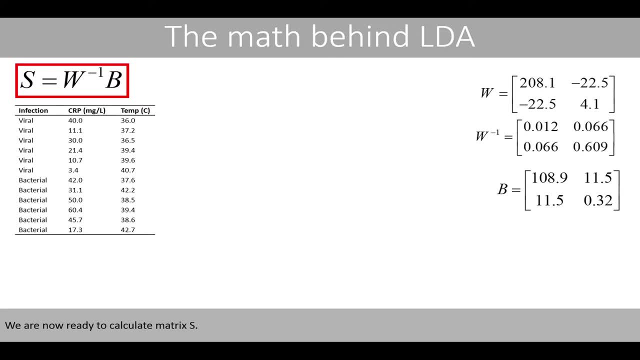 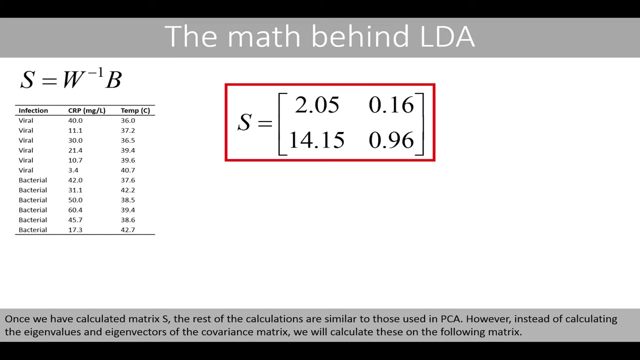 We are now ready to calculate matrix S. We calculate matrix S by multiplying the inverse of the pooled within-group covariance matrix by the between-group covariance matrix. Once we have calculated matrix S, the rest of the calculations are similar to those used in PCA. 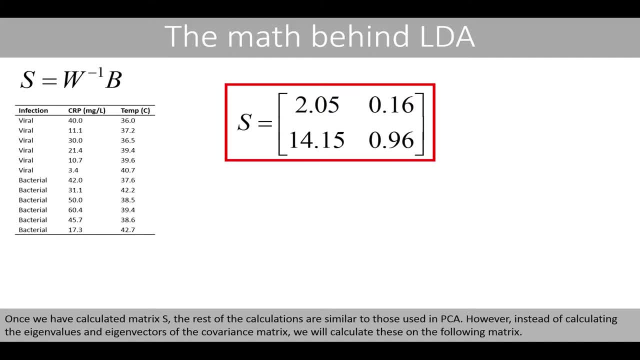 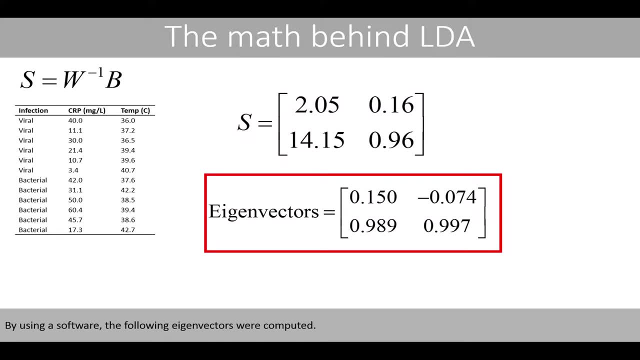 However, instead of calculating the eigenvalues and eigenvectors of the covariance matrix, we'll calculate these on the following matrix By using a software. the following eigenvectors were computed: This is the first eigenvector of matrix S, whereas this is the second eigenvector. 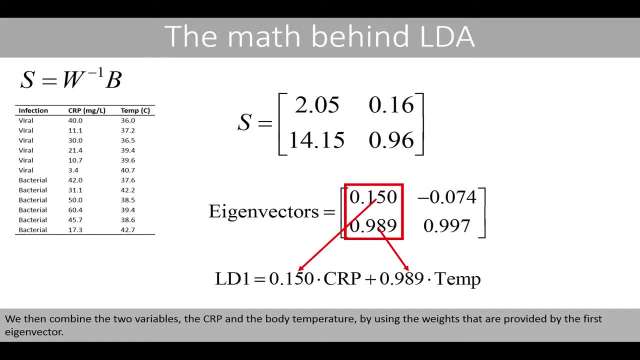 We then combine the two variables, the CRP and the body temperature, by using the weights that are provided by the first eigenvector. By using this equation with the given weights, we can calculate the discriminant scores that will show the best linear separation between the groups. 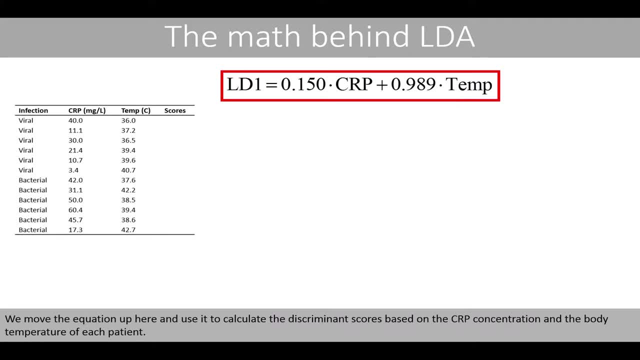 We move the equation up here and use it to calculate the discriminant scores based on the CRP concentration and the body temperature each patient. These are the calculated unstandardized scores. We'll now rescale these weights so that they correspond to the weights or loadings that are commonly 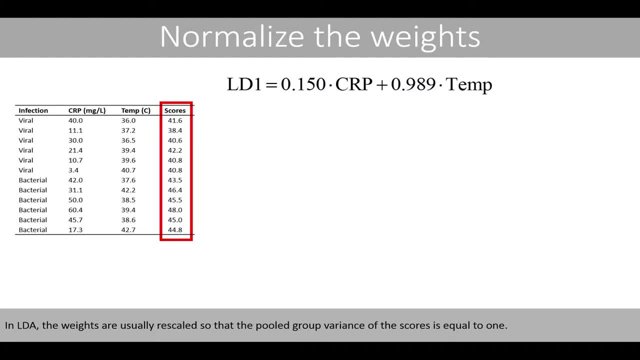 shown by most statistical software tools. In LDA the weights are usually rescaled so that the pooled group variance of the scores is equal to 1.. Let's calculate the variance of the scores for the virus group. The variance of these scores is about 1.6, And the variance of the scores for the bacteria group is 2.37.. 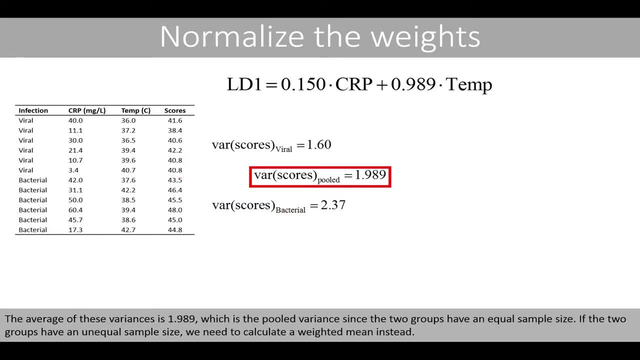 The average pause is 1.989, which is the pulled variance, since the two groups have an equal sample size. If the two groups have an unequal sample size And the average time wise is 14 minutes, So its very easy to estimate where this variance. 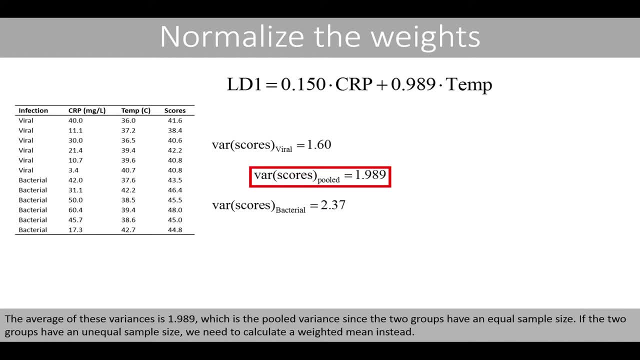 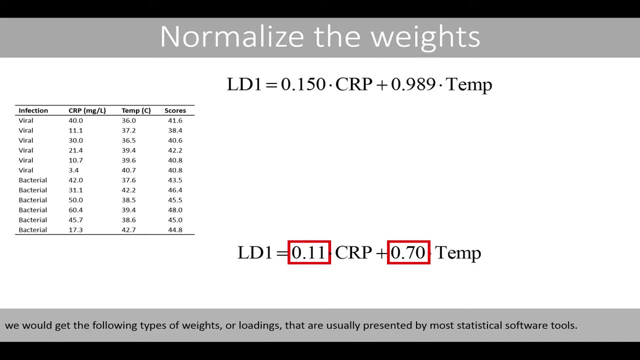 we need to calculate a weighted mean instead. If we now divide the weights by the square root of the pooled variance, which corresponds to the pooled standard deviation, we would get the following types of weights or loadings that are usually presented by most: 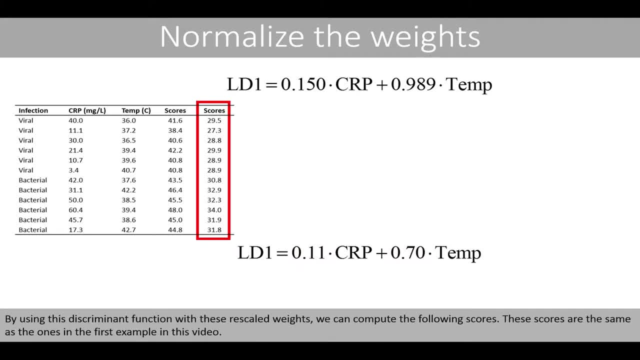 statistical software tools. By using this discriminant function with these rescaled weights, we can compute the following scores. These scores are the same as the ones in the first example in this video. If we now calculate the variance of the scores for each group, 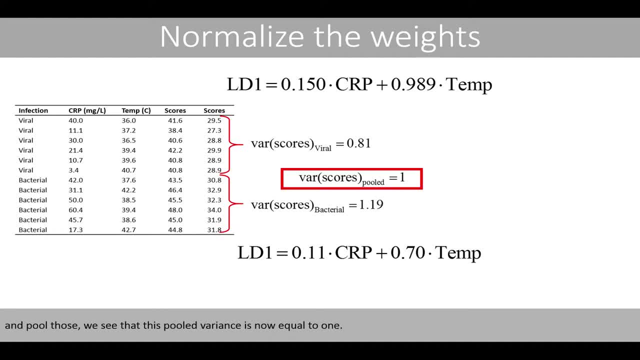 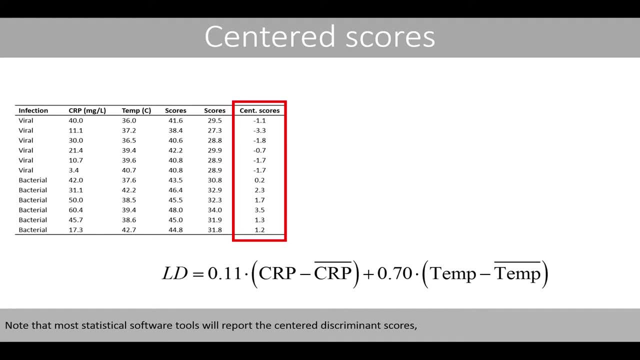 and pool those, we see that this pooled variance is now equal to one. Note that most statistical software tools will report the centered discriminant scores, which can be calculated based on the following equation, where we first subtract the means from the original values: 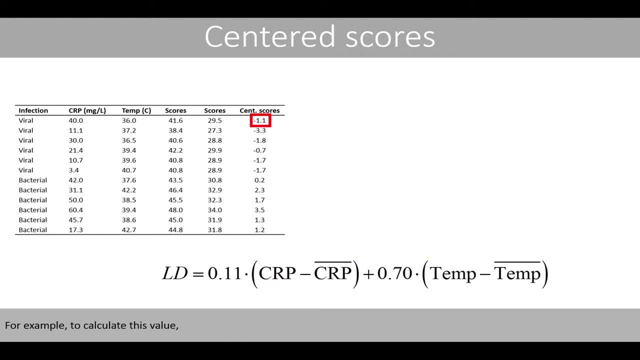 For example, to calculate this value, we plug in the two measurements for this person and the means of the two variables. By doing this, the score is calculated to about minus 1.1.. Finally, we will have a look at the so-called standardized discriminant function. 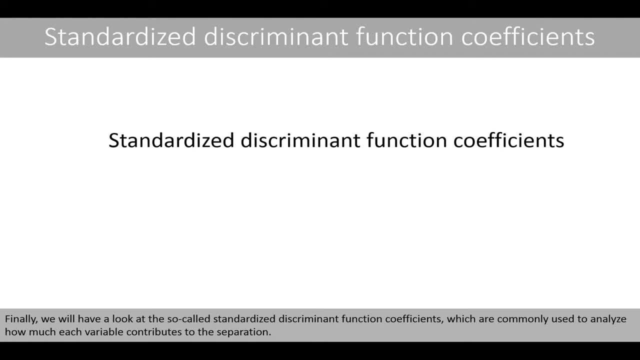 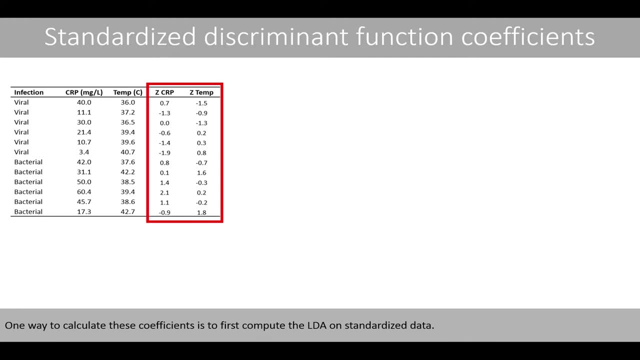 coefficients, which are commonly used to analyze how much each variable contributes to the separation. One way to calculate these coefficients is to first compute the LDA on standardized data. To standardize a variable, we usually subtract its mean from the original values and divide by the square root. 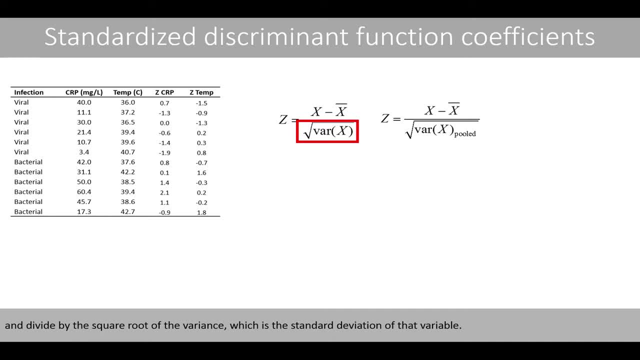 of the variance, which is the standard deviation of that variable. In contrast, for LDA, we divide by the square root of the pooled variance of the groups for that variable. If we use this equation, we will get the following standardized variables: 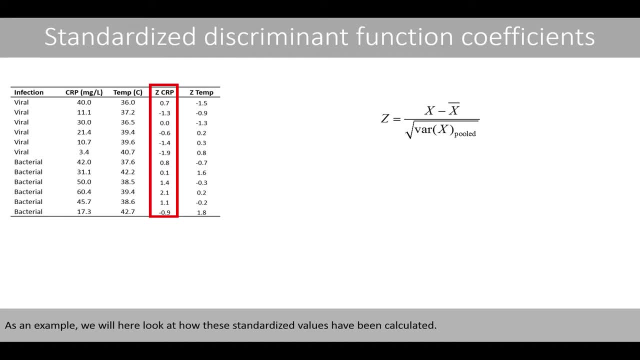 As an example, we will here look at how these standardized values have been calculated. We first need to calculate the mean of the CRP variable, which is 30.3.. The variance of the CRP for the virus group is 188.3, and the variance 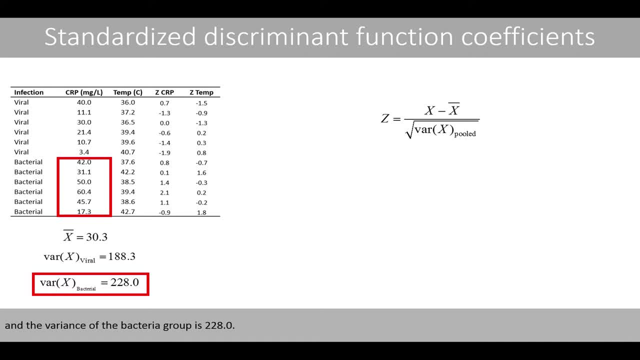 of the bacteria group is 228.0.. We can now pool these two variances and since the sample sizes are equal between the groups, the pooled variance is simply the mean of these two variances. We see that the pooled variance is 208.1.. 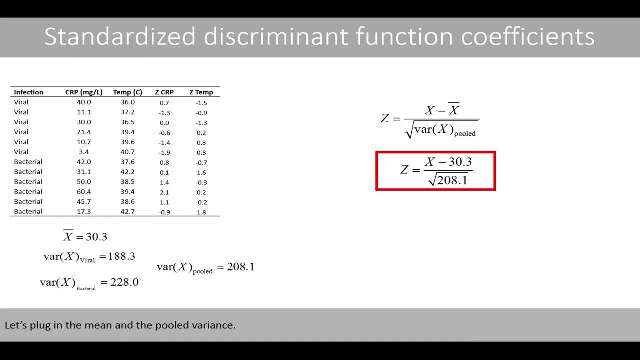 Let's plug in the mean and the pooled variance As an example. we will here calculate the standardized CRP value for person number 1.. We see that the calculation results in a standardized value of about 0.7.. We now use these values to compute the scores.